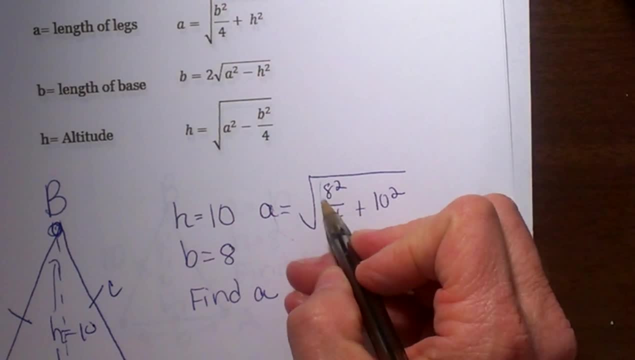 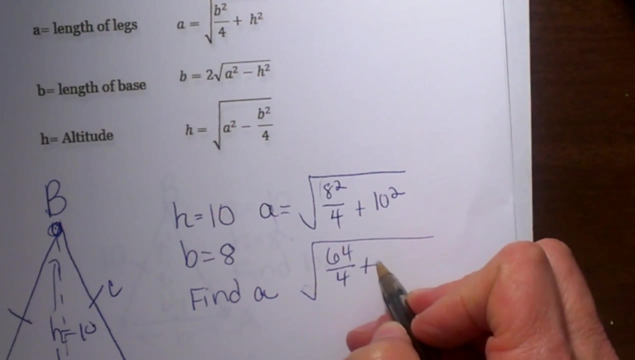 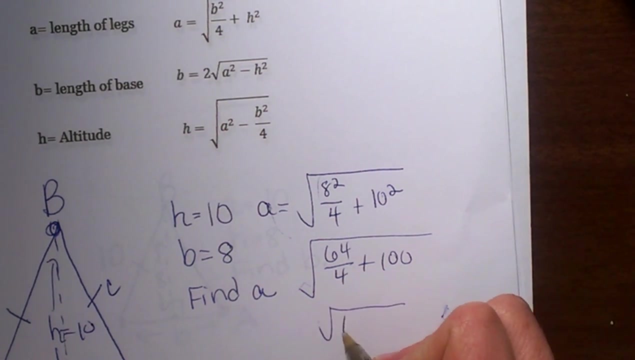 So all we have to do now is simplify this. So let's take this 64.. 8 squared is 64.. So 64 over 4 plus 100 for 10 squared, and 64 divided by 4 is going to give me 16.. 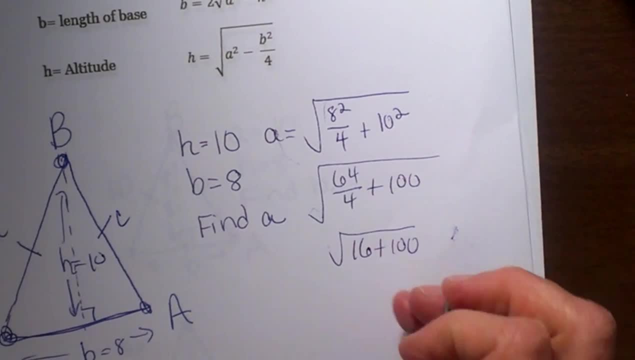 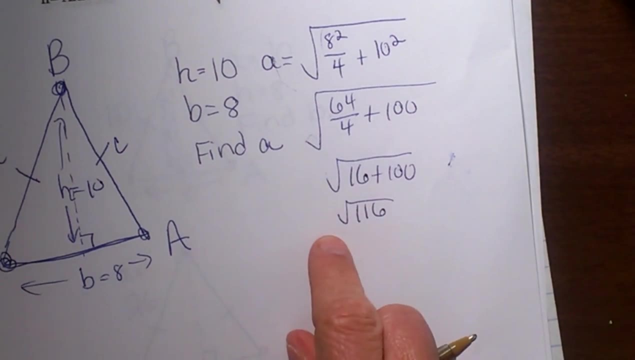 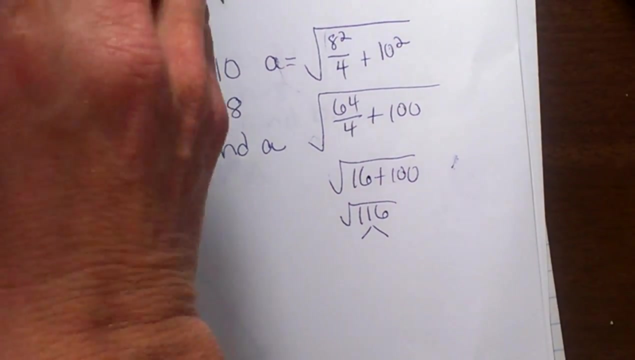 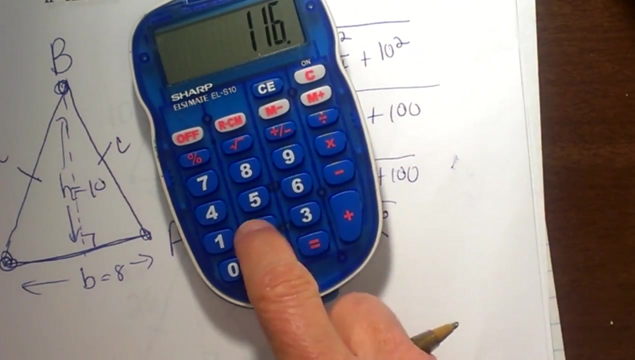 16 plus 100 will give me 116. From here. that is my answer and I can write that as a decimal. but typically what we like to do is go ahead and simplify that. So let's see If I divide 116 by 2 to simplify this radical. so I am going to take 116 divided by 2 and 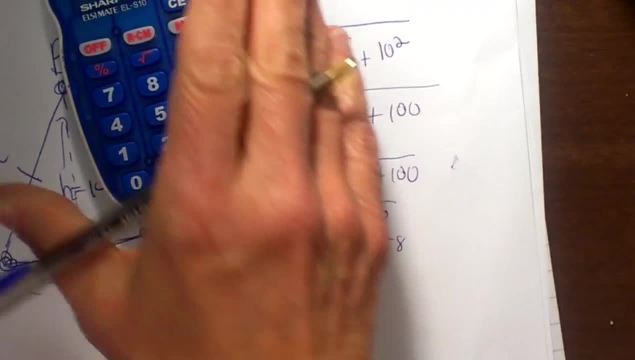 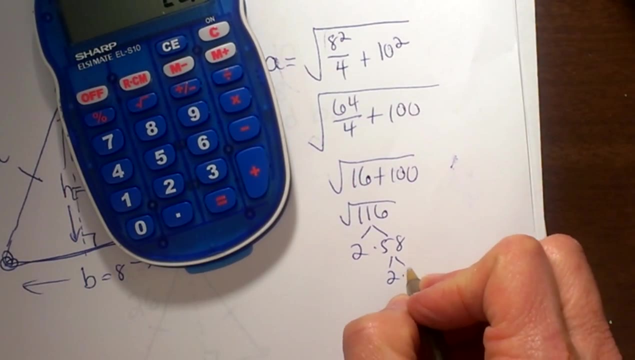 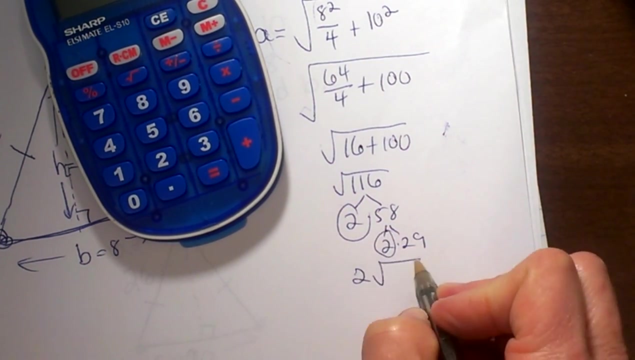 that is going to give me 58, and 58 is even so. let's divide that by 2 again and that gives me 29. 29 times 2.. Once I get a pair, I can take it out of the radical. so this is going to simplify to 2. 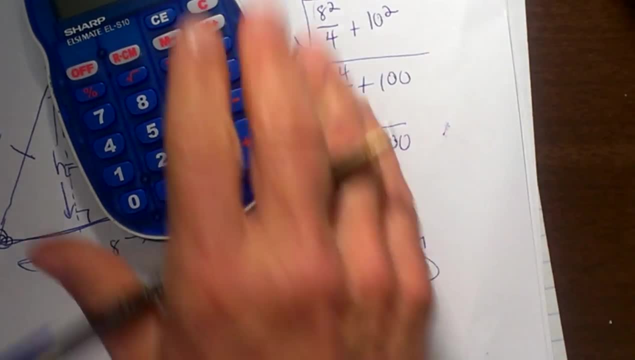 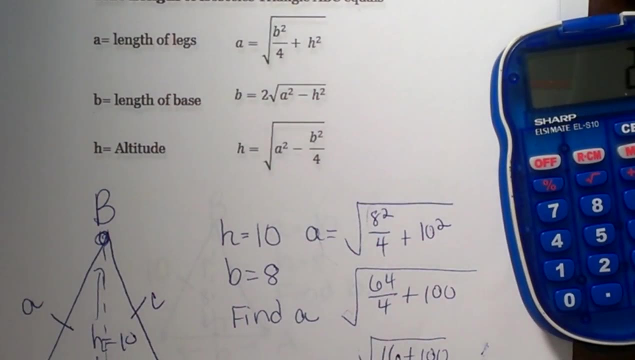 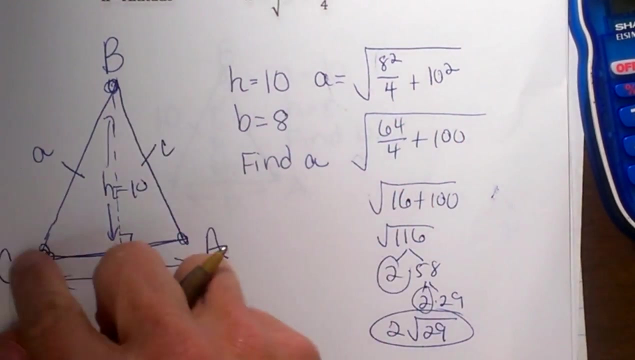 square root 29.. That is how long. That is how long the base of this triangle is, using this little formula. So hopefully that was kind of helpful. Another way to look at that is just to use the Pythagorean Theorem. So if I split this triangle, I have an isosceles triangle here, and I know this. altitude cuts. 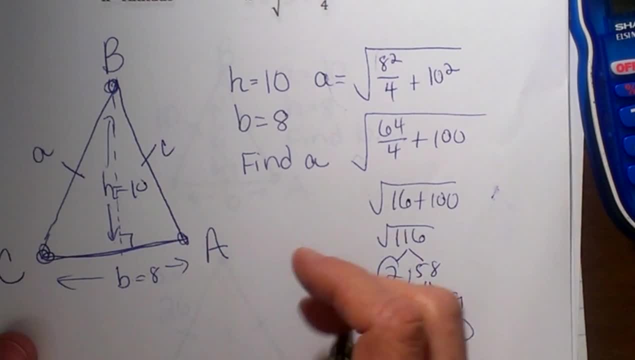 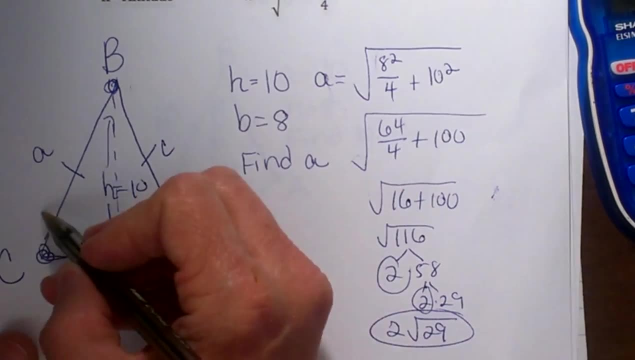 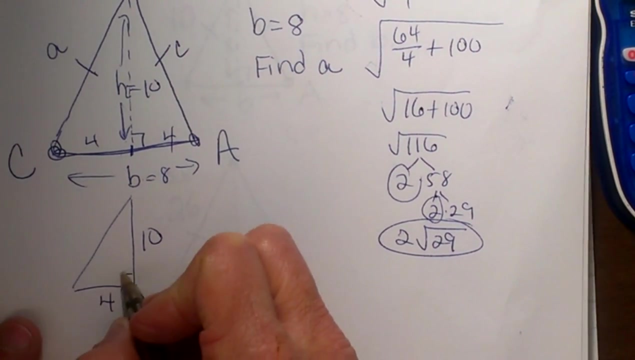 this base in half. So if this base is 8, I can cut it in half and make that 4 on this side and 4 on this side. Then I can isolate this little right triangle right here. So my height would be 10 and my base would be 4 and I would have to have a right angle. 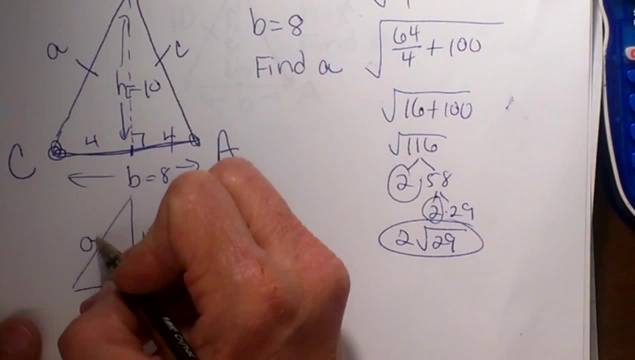 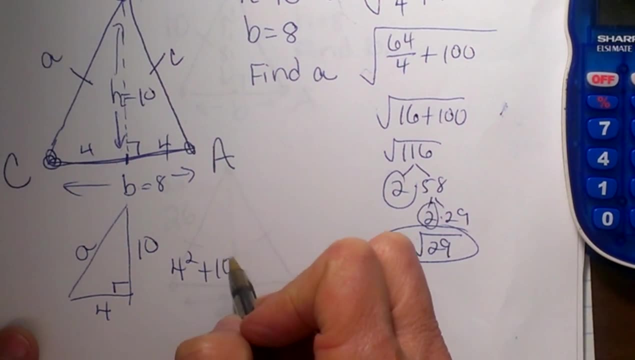 here. Then I can just use the Pythagorean Theorem to find this side a over here. So I can take 4 squared plus 10 squared and that is 16 plus 100 or 116 and that is going to equal c squared. 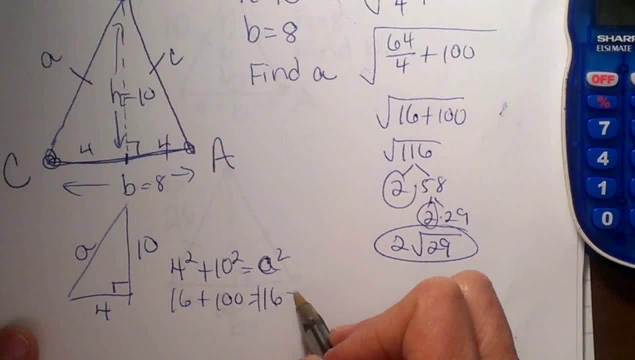 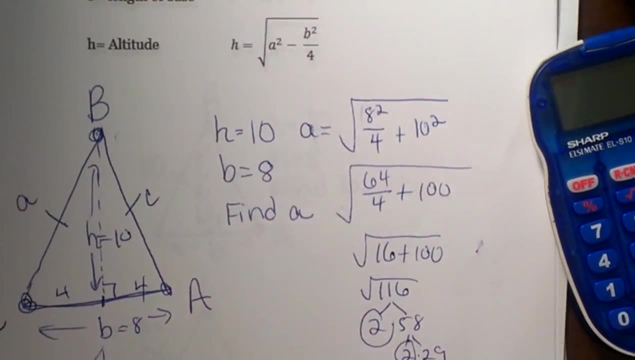 Or a squared, And I am going to take the square root of that, which we know is 2 square root 29.. So just another way to think about that. I hope this video was helpful on using our little shortcut formulas.